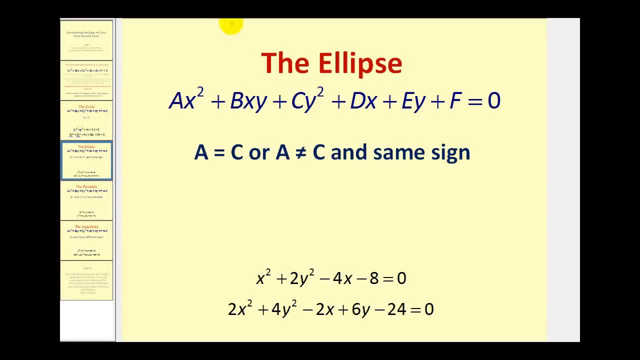 equal c, but they have the same sign. we would have an ellipse. Now it may seem like this is overlapping with the conditions for a circle, And it is because all circles are ellipses. So the coefficients of the x squared term are not all equal to zero, So the coefficient 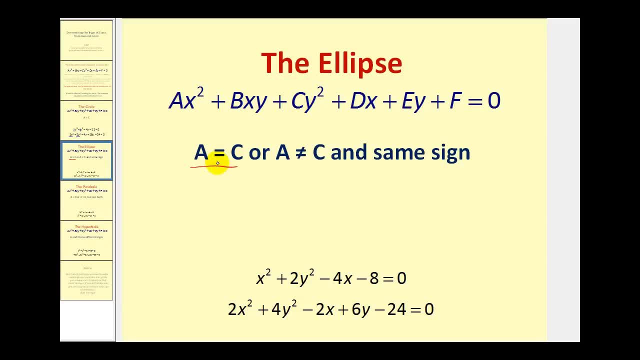 of the x squared term equals the coefficient of the y squared term equals the coefficient of the y squared term. And the y squared term can equal each other or not, but they do have to have the same sign And if this is the case, we will have an ellipse. So this: 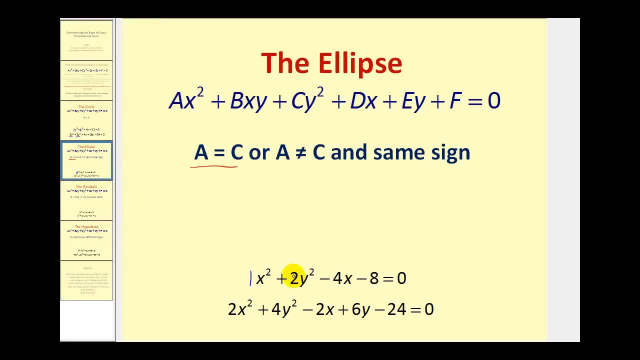 first example: we have a equals one and c equals two. They're both positive. Therefore we have an ellipse. And the second example: we have a equals two and c equals four, both the same sign. Therefore we have an ellipse For a parabola. we must have a equals zero. 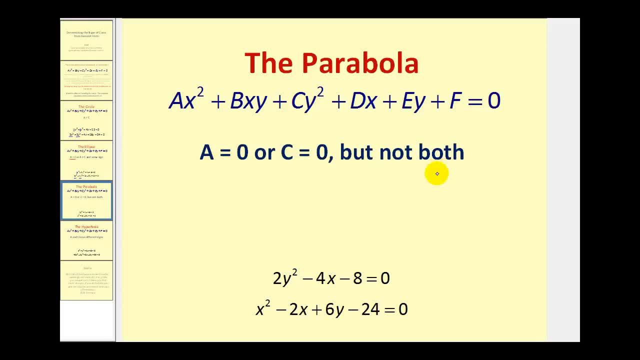 or c equals zero, but not c equals zero. So we have a equal to zero and c equals zero. So what that means is either there's no x squared term or there's no y squared term, but there must be one of them. This first example: we have a y squared term, but no. x squared term, so a would equal zero, but c is equal to two. In the second equation we have a equals one and there's no y squared term, so c would equal zero. The last conic we'll look at is the hyperbola. 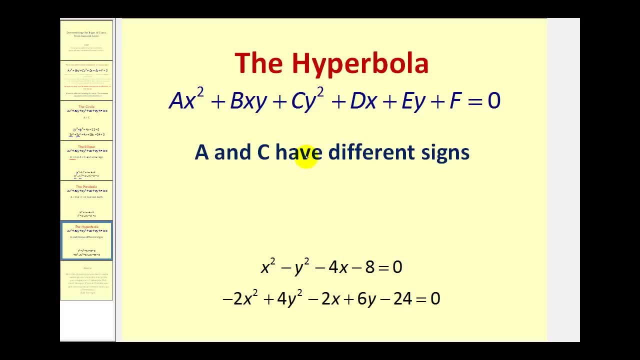 And the equation will always be a hyperbola if a and c have different signs, or the coefficients of the x squared term and the y squared term have different signs. So in this first example we have a equals one and c equals negative one. Therefore, we have a hyperbola In the 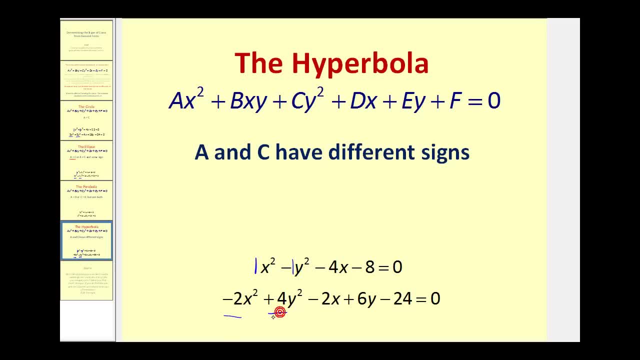 second example: we have a equals negative two and c equals positive four, which have different signs And therefore we have a hyperbola. There are several other videos on conic sections dealing with graphing the conics in general and standard form. This: 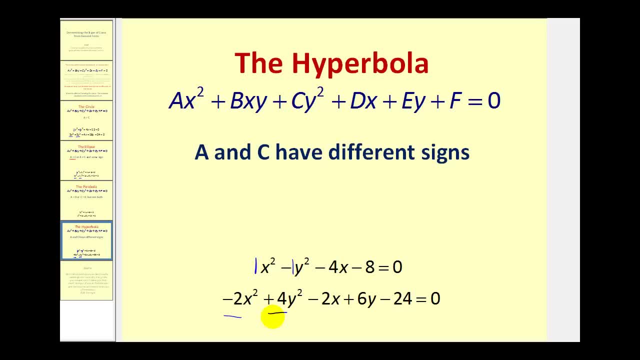 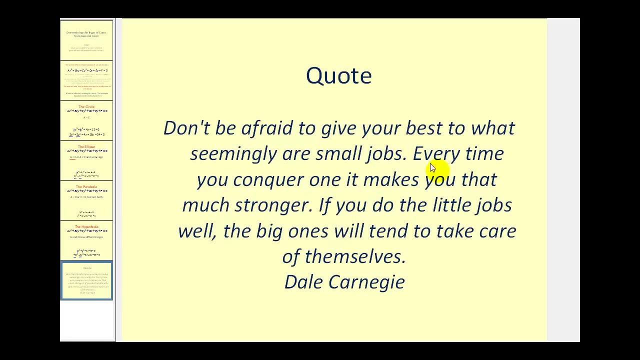 video just dealt with identifying what type of conic we have from the equation in general form. I hope you found it helpful and thank you for watching. Thank you for watching.